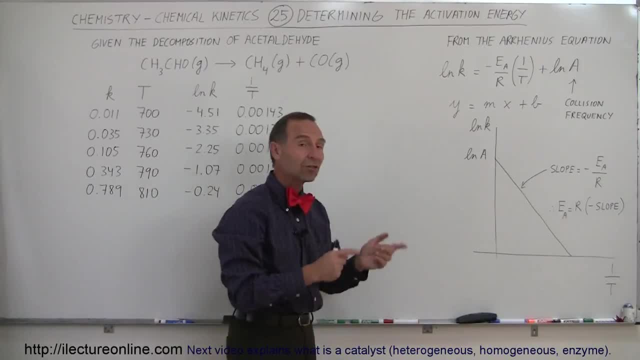 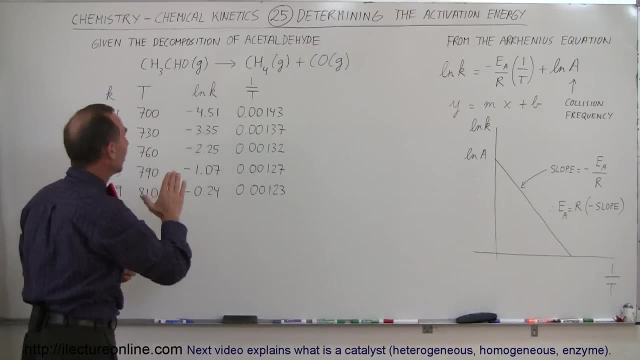 a from a from a from a reaction, we can actually figure out what that activation energy is. So let's determine the slope from this, from this data here- but notice the data of course is taken out is taken in terms of the reactant constant and the temperature. we have to take the 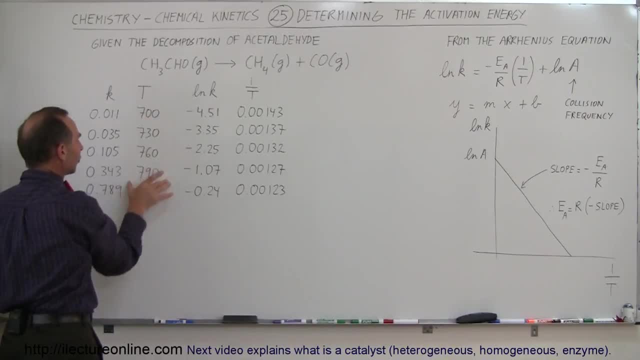 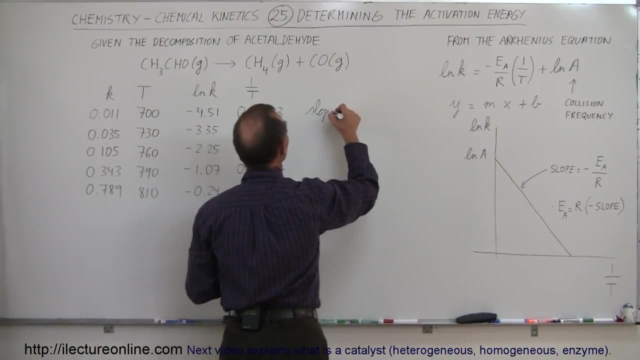 natural log of that. which are these numbers right here? and we have to take the inverse of the temperature. which are those numbers right here? So here we can see that the slope can be determined. the slope is equal to the rise divided by the. 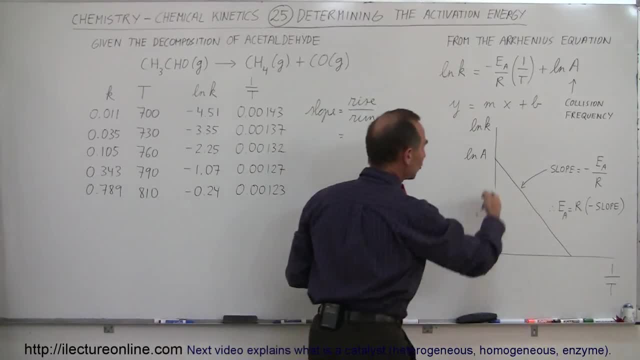 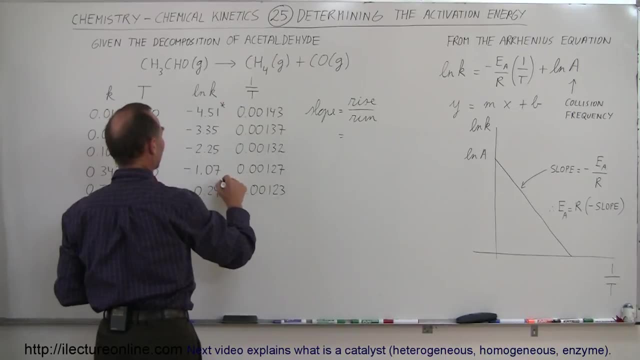 run and of course the rise would be the change in the vertical distance, that would be, the change in natural log of k. So let's take this value right here and let's take this value right there and take the difference of the two that 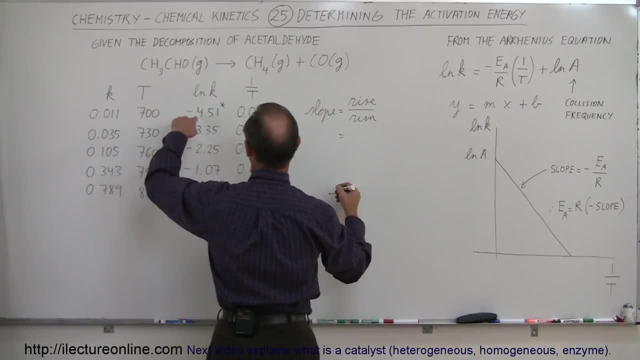 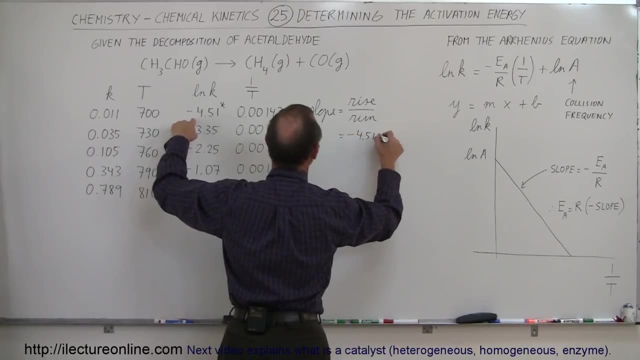 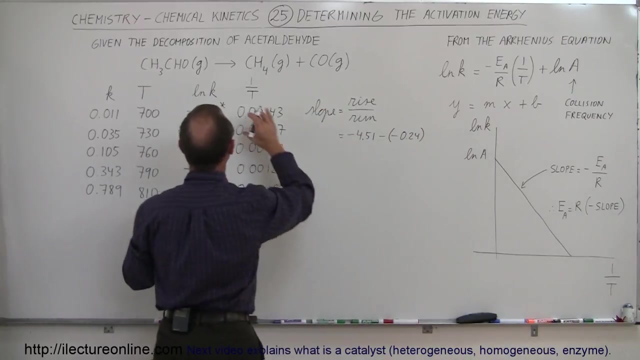 would be the change. So that would be the initial value right here minus the final value. you could do it either way. so it would be minus 4.51 minus the minus 0.24, that would be the natural log of k at this temperature minus the natural log of k at this temperature. 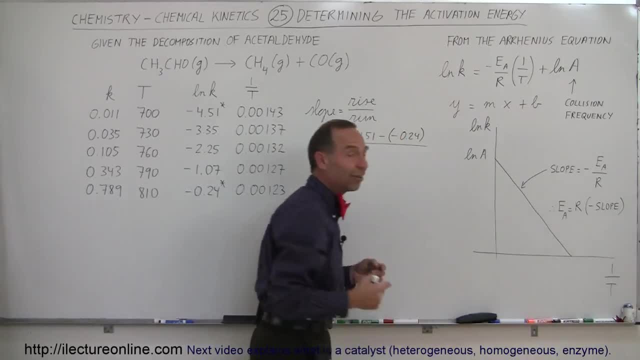 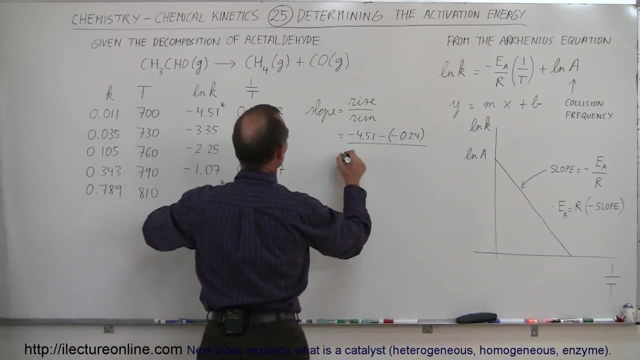 right there and we divide that by the run, which is the horizontal distance, it's the difference in one over the temperature. but since we went this number minus this number, we have to go this number minus this number in the denominator, so it would be 0.00143. 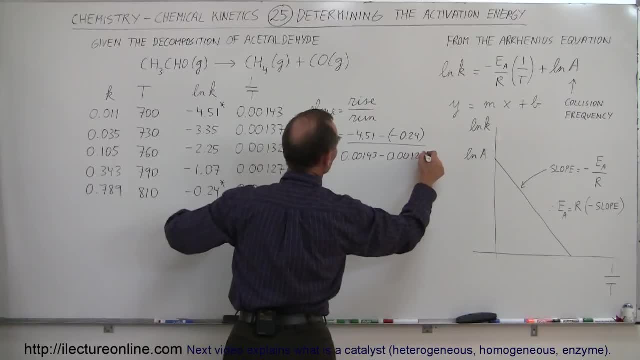 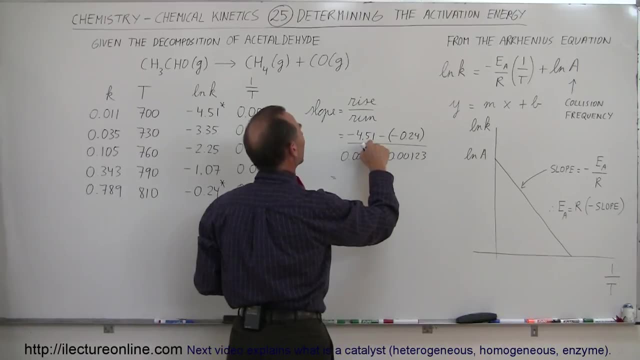 minus 0.00123, and so this is equal to. that becomes a positive. add a positive 0.24 to that. that would be- hmm, actually it's like a subtraction- that would be minus 4.27, because. 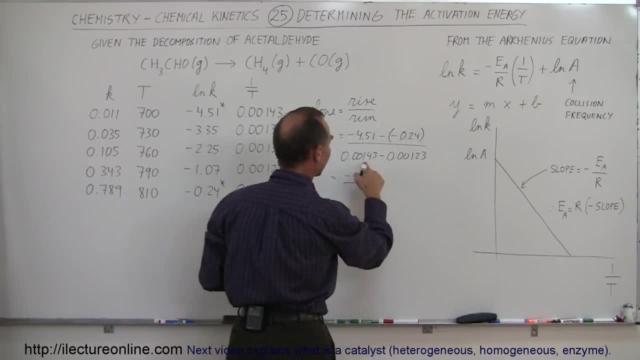 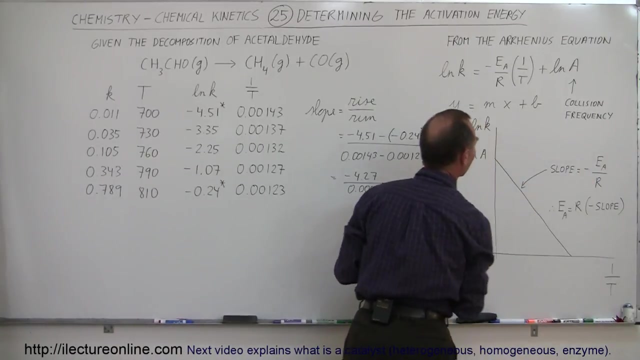 24 plus 27 is 51, divided by, and the difference between these two looks like it's it's 0.00020.. All right, so that's equal to the slope. and notice, by the definition, the slope is equal to the activation energy divided by the gas constant. so this must be equal. 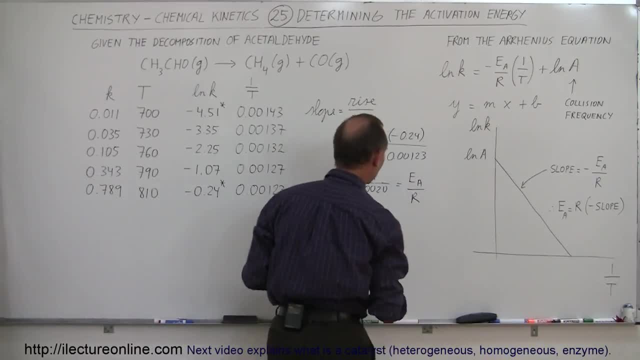 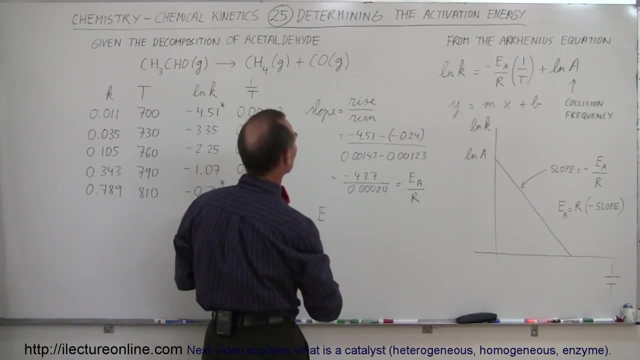 to the activation energy divided by the gas constant, and that means that the activation energy E- and of course let's see here the slope- is the negative of that. can't forget that negative sign. So notice that this negative sign will then, of course, cancel out this negative sign. 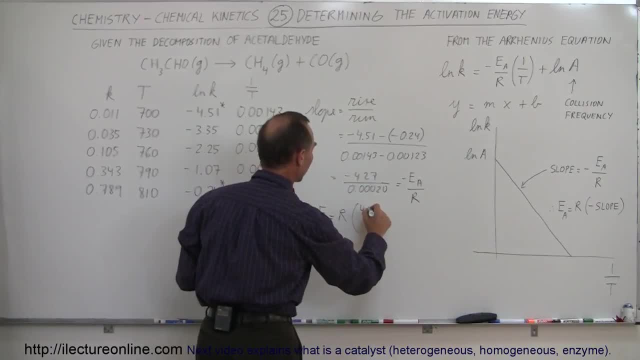 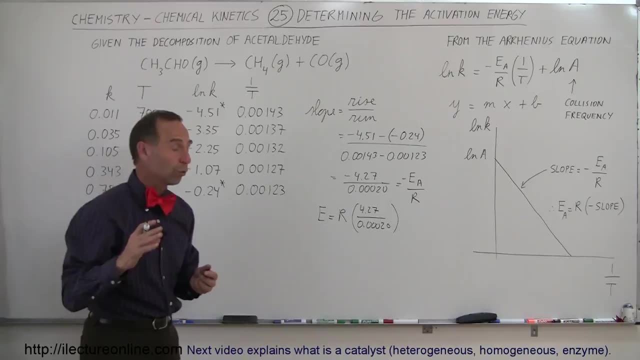 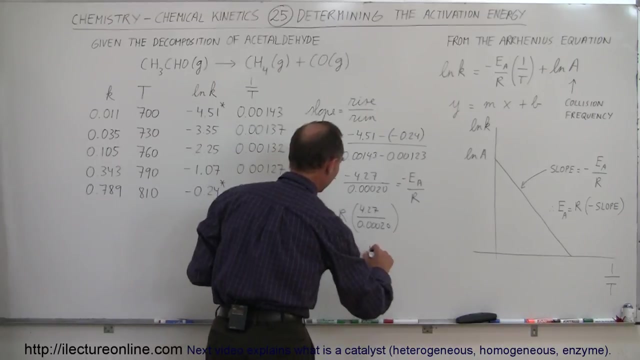 and the activation energy is equal to the gas constant times its ratio of 4.27 divided by 0.00020, and since, of course, the gas constant is in terms of joules, the activation energy will also be in terms of joules, because this is 8.315 joules per mole times kelvin. 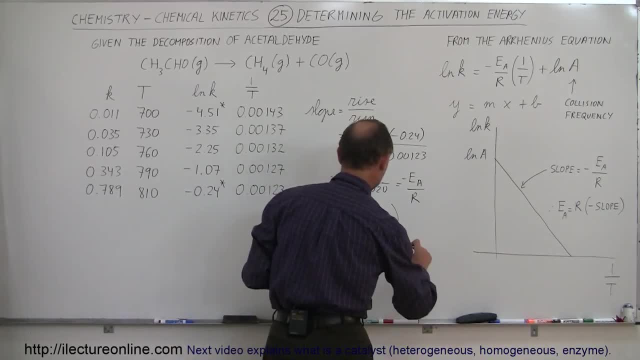 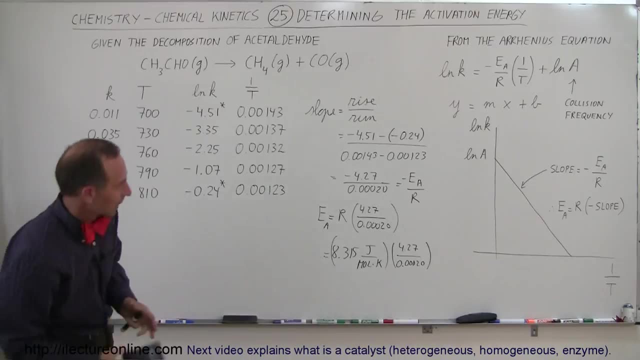 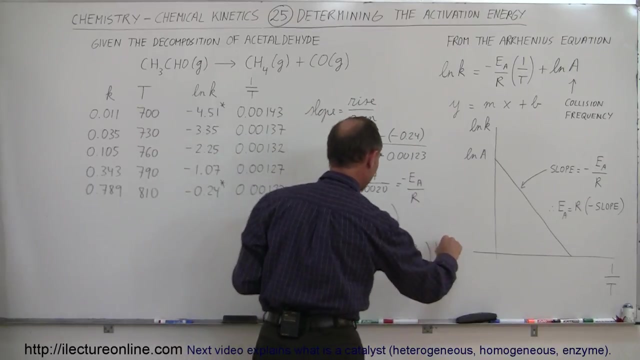 times 4.27 divided by 0.00020.. Okay, And that will give us. let's see here: this is the change in the one over the temperature. so that would be temperature, that would be kelvin in the numerator. and if we do this, 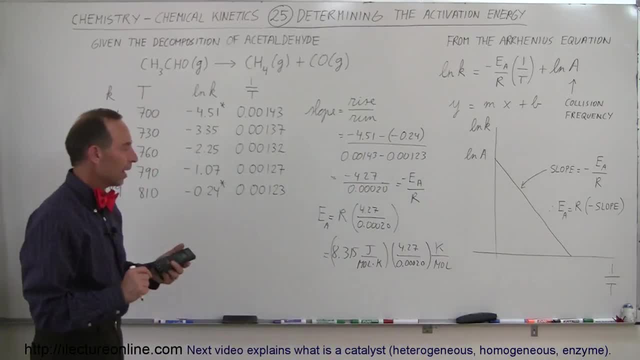 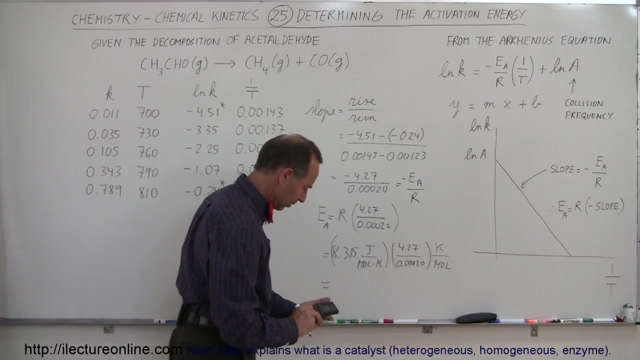 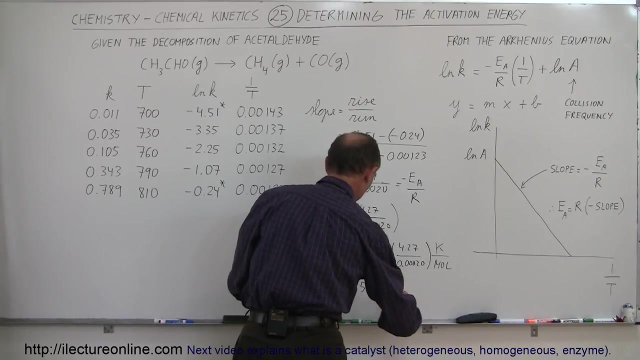 per mole. we get moles in the denominator, so we get 8.315 times 4.27. divided by 0.0002 equals, and the activation energy is 0.0002.. Okay, So the activation energy is 177,525 joules per mole, or 177.5 kilojoules per mole. 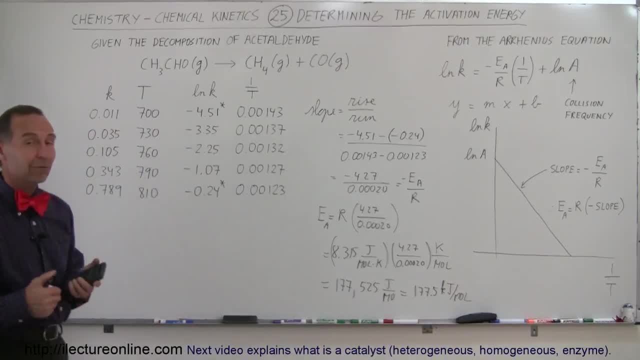 And that is actually a pretty interesting way to find the activation energy. Of course you can't just do that via a theoretical equation. you have to read in the rate constant. as you're watching the reaction, You have to measure the temperatures when it happens, so you can see that the rate of 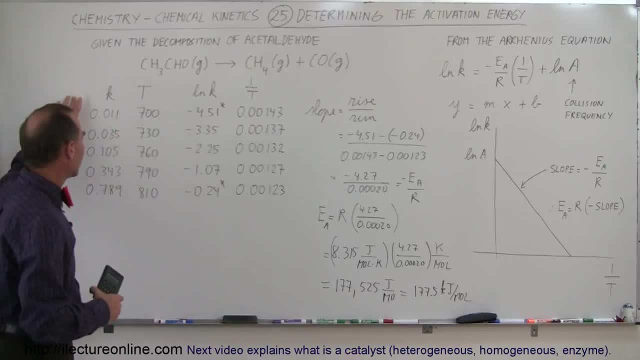 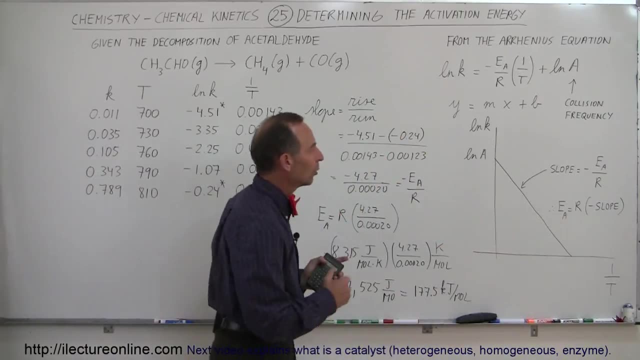 the reaction changes with the temperature. You take the natural log of the reaction rate constant. you take the inverse of the temperature. from that you find the slope of that equation. realizing the slope is equal to the negative of the activation energy divided by the gas constant. and then, of course, you equate the 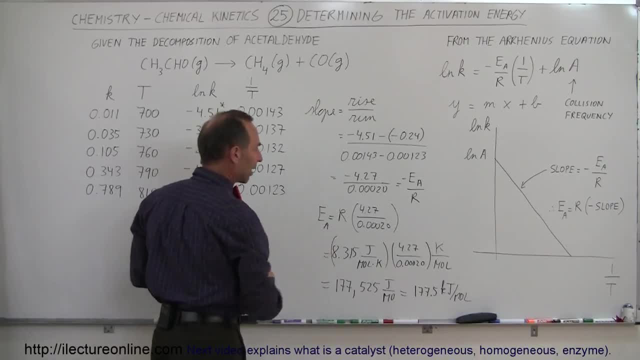 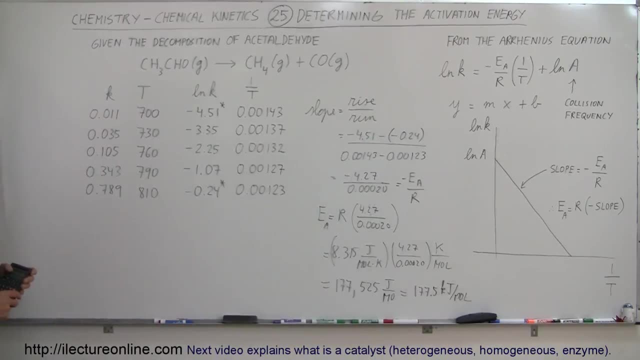 slope from the numbers. you set, that equal to the activation energy times, the gas constant, and there you get the result: A pretty slick method and it's very effective. Thank you. 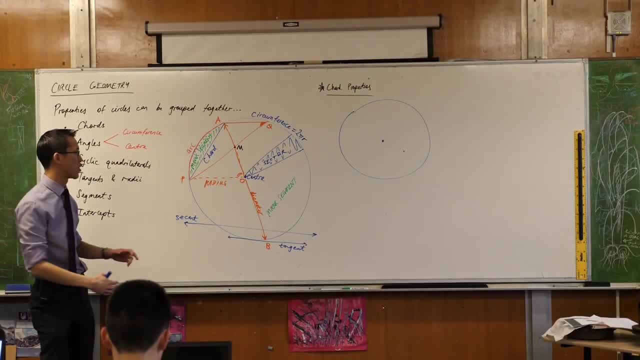 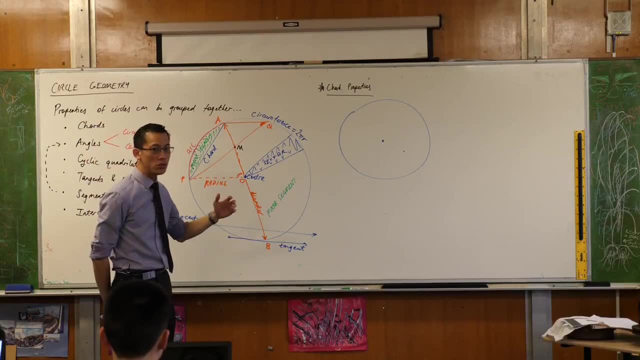 You've got a circle- any circle. These ones can be a bit smaller because we're not going to put such a huge number of things on them. okay, Draw a circle, any circle, and then what I'd like you to do is: onto your circle, I'd like you to draw.